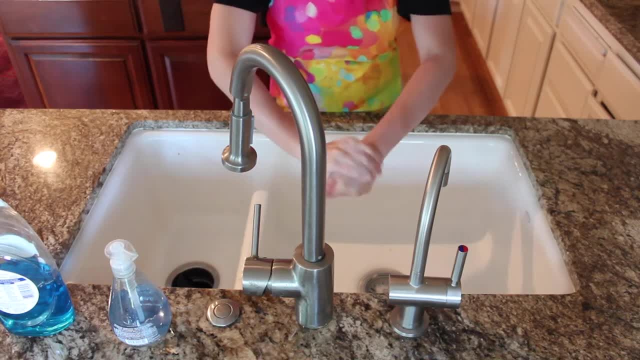 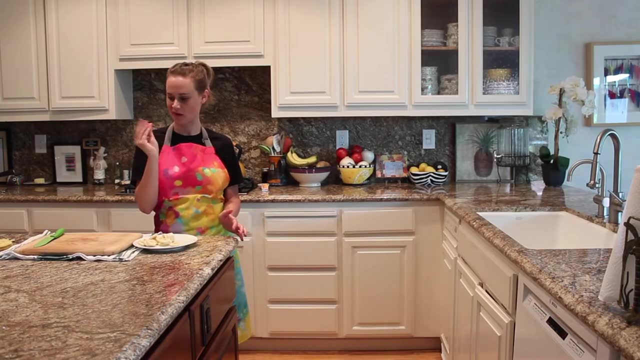 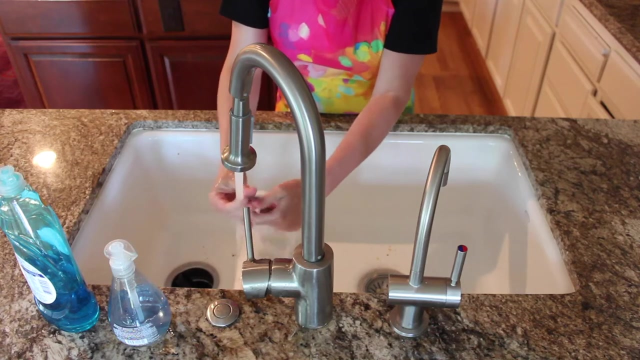 sure I can sing the entire alphabet before finishing up. You get the point. Make sure to wash your hands every time you touch your mouth or face. If you're using a tasting spoon, make sure to wash it before using it again. Clean as you go. This doesn't just make your parents happy, but it's also for. 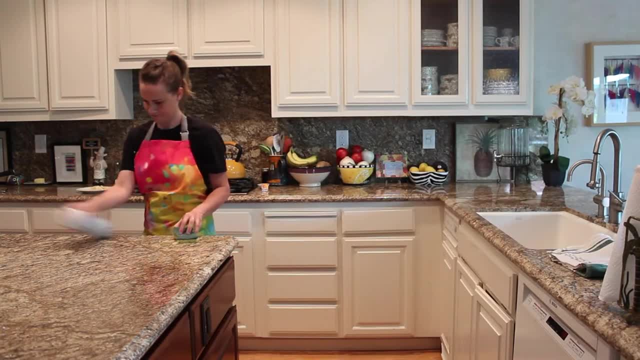 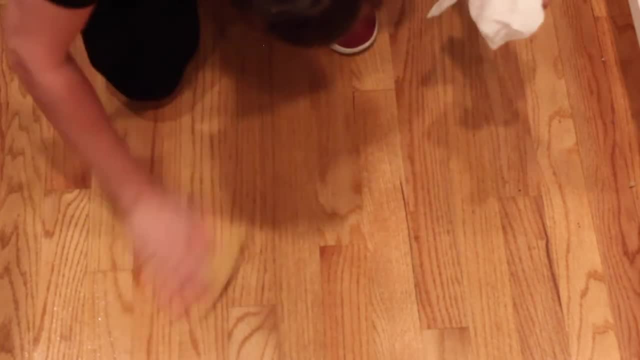 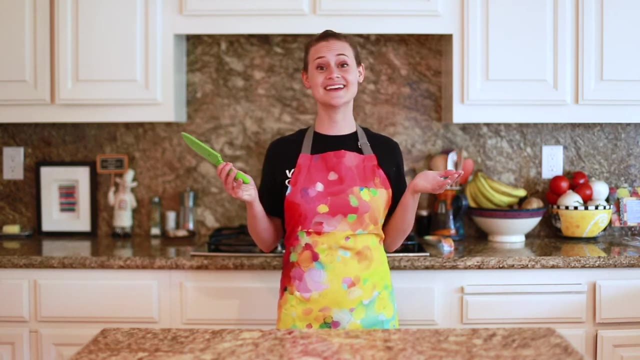 safety. It is safer and easier to work in an uncluttered space and clean your kitchen. Clean as you go avoids accidental cross contamination by ingredients like raw eggs. Let's talk about using knives in the kitchen. It's easy. All you have to do is remember. 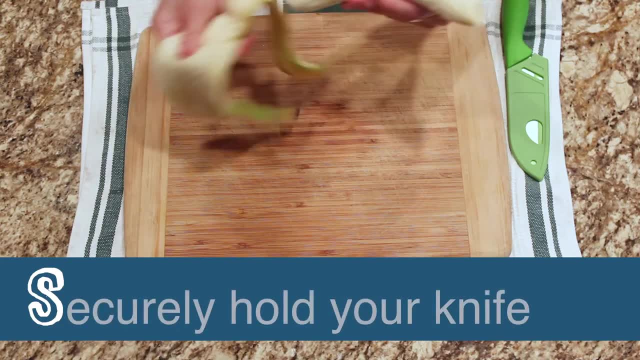 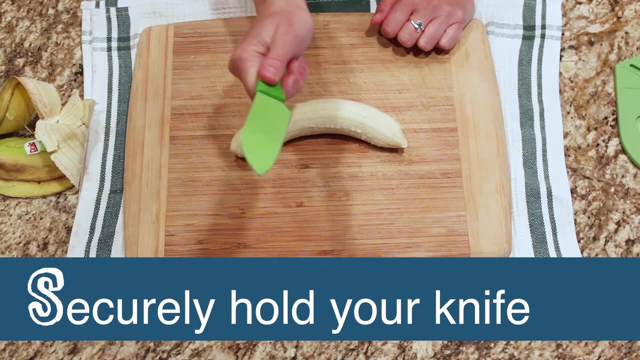 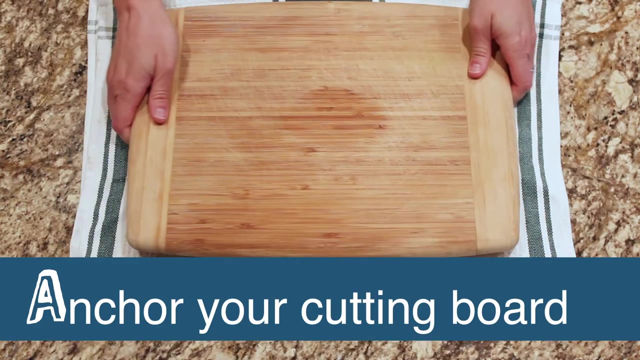 to spell out the word safety S: Securely hold your knife. You can do this by placing four fingers on one side and your thumb on the opposite side of the handle. A Anchor: your cutting board. Always use a cutting board. If necessary, place a damp towel underneath to prevent it from 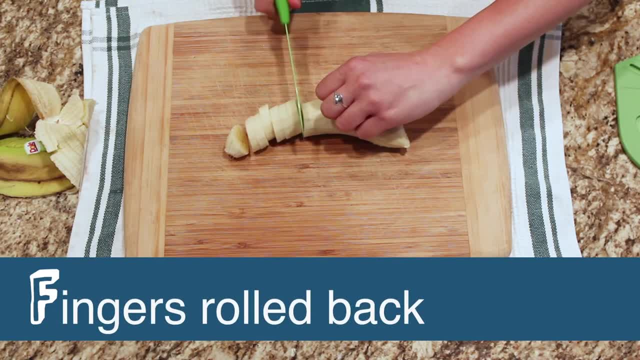 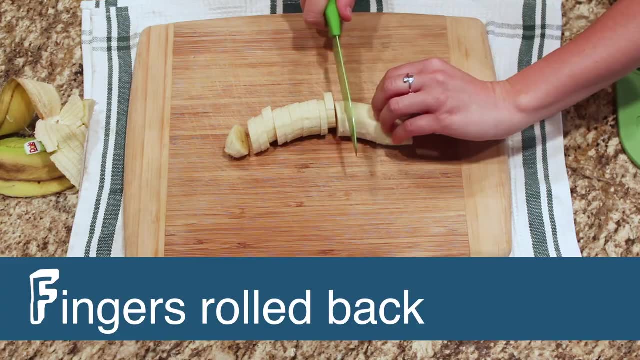 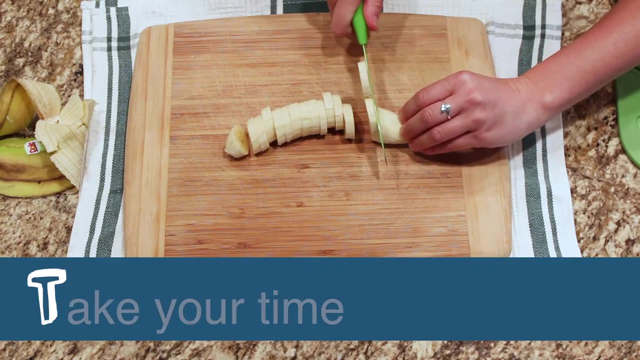 sliding around. F Fingers rolled back. Create a bear claw grip to hold the food being cut. This keeps fingertips away from the blade. E Eyes on the knife: Always watch what you are doing. T Take your time, Don't rush. 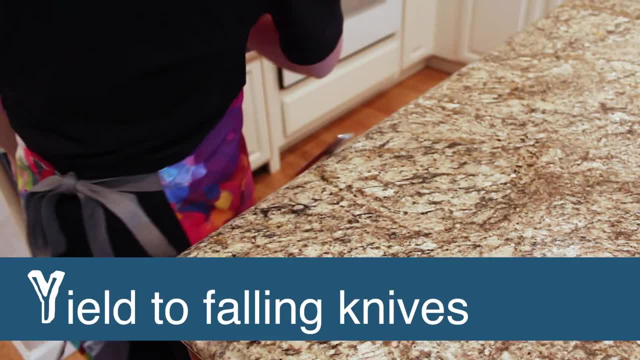 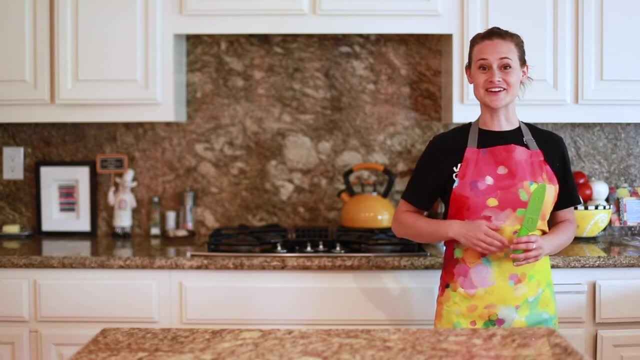 And Y Yield to falling knives. If you drop a knife or knock it off the table, don't try to catch it, Just step out of the way and let it fall. As long as you are practicing safety, you can innovate safely while using a knife in. 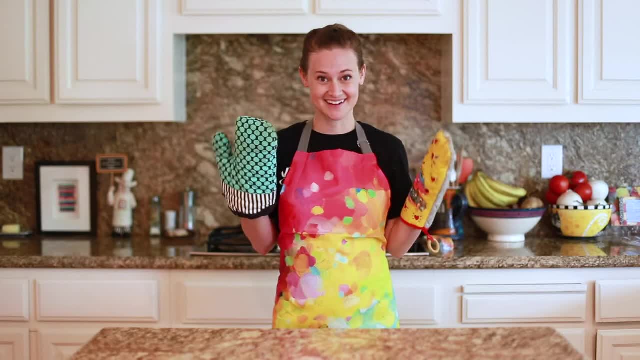 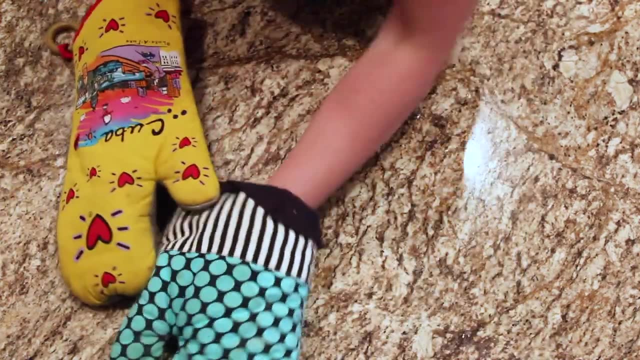 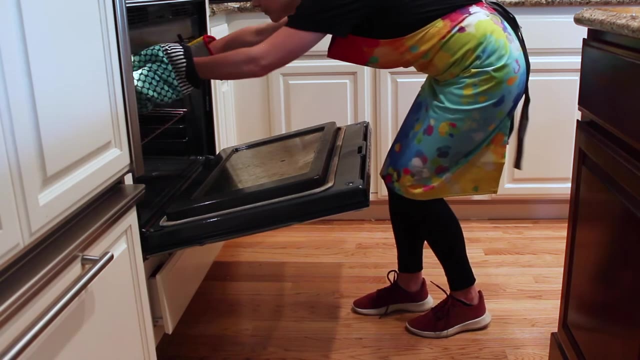 the kitchen. Let's talk about heating elements like ovens, toaster ovens and stoves. Always use an oven mitt when putting things into the oven, even if the pan isn't hot. You don't want your hand to accidentally touch a hot part of the oven as you are putting it. 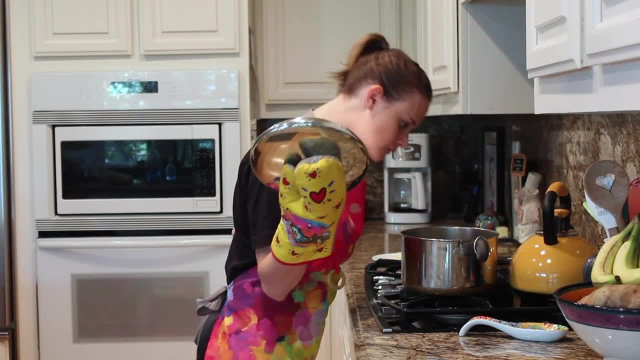 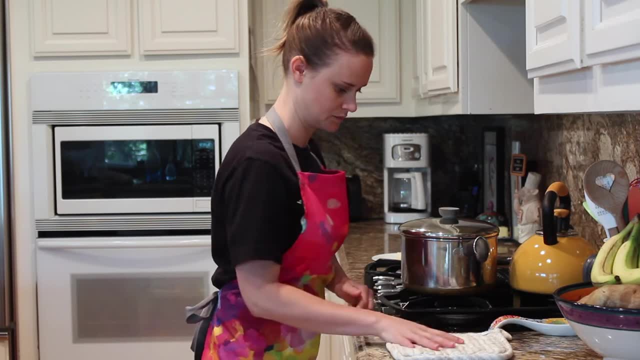 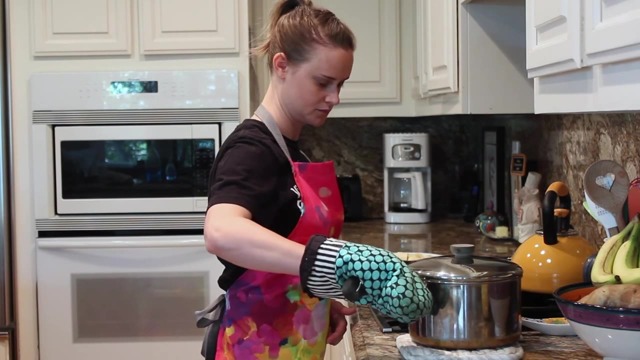 in. Always use an oven mitt, potholder or towel to carry and hold items on or coming from a hot surface. Always put hot pans on heat-proof surfaces, like hot pads or towels. Don't put them on anything plastic which can melt or crack. Some countertops, like granite, are heat resistant.